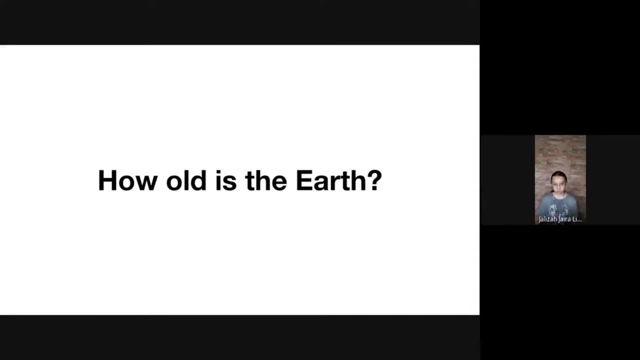 pause for a few seconds to ask you to ponder about the age of the Earth. You're right: it's older than any of our grandmas, or all of our grandmas combined. So it's actually 4.6 billion years old. Wowza, Imagine how many zeros are there? Yep, a lot. Now one formation. 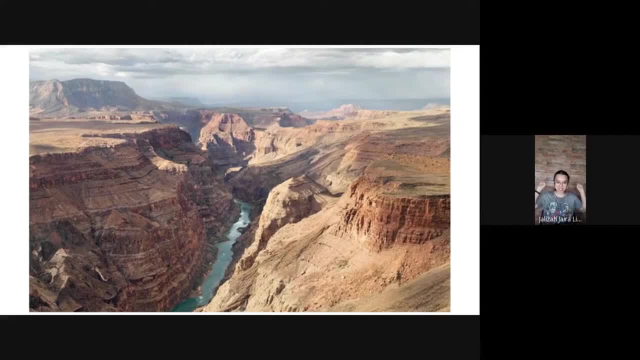 that actually captures the whole history of the Earth is the Grand Canyons. Now, if you would look at the Grand Canyons, you'd see that they're actually 4.6 billion years old. And they're 4.6 billion years old. Now, if you look at the photo and if you could actually see it clearly. 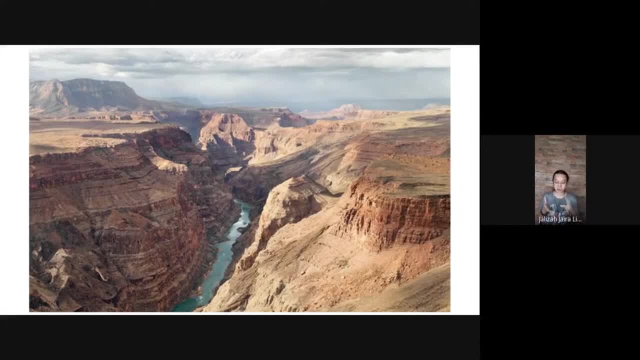 there are rock strata or rock layers. There are many rock layers there. So, with that, each and every rock layer actually tells a different story and oftentimes a different time period, Because, as we may know, rocks tend to take thousands, millions of years to actually form. So with that, the 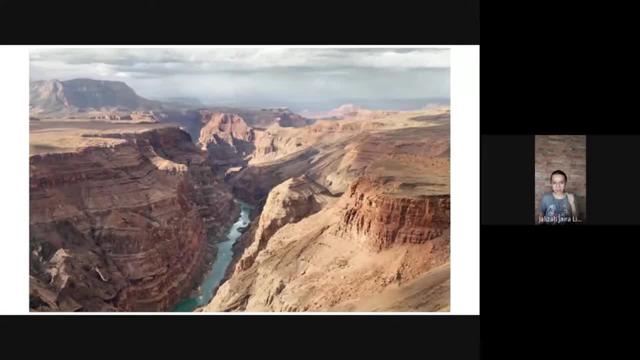 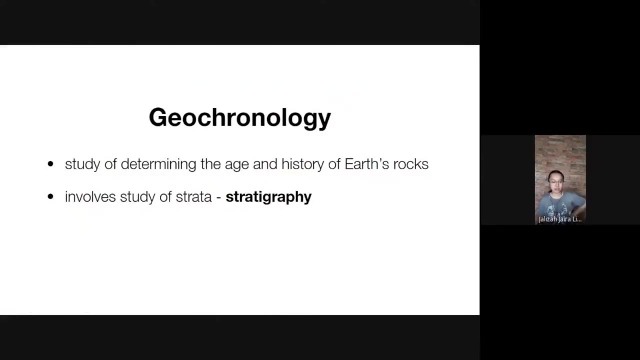 different rock layers found at the bottom of the Grand Canyon may have actually been here at the start of the Earth's formation or during the start of the formation of the Earth, And that one particular field of study that actually tries to tell us about the age and history of the Earth. 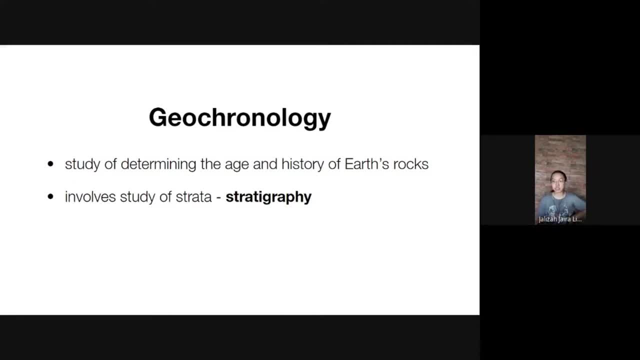 is geochronology And it tries to study strata or the rock layers that are present around us, And that the study of this strata is actually your stratigraphy. So we're trying to understand rock layers. So, when it comes to stratigraphy, 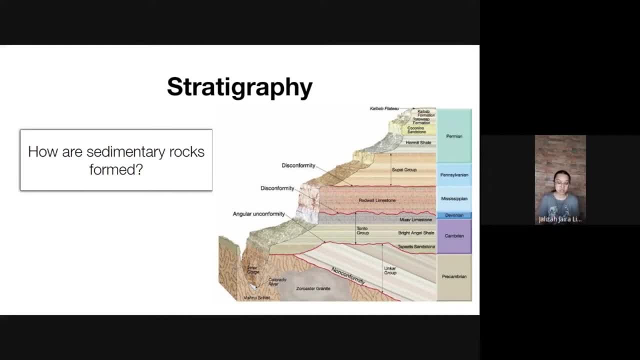 it tries to answer the question: how are sedimentary rocks formed? Now, if you will remember, rocks undergo weathering, erosion, eventually transport, deposition and eventually they start to plump together, forming very different layers. So your Grand Canyon is actually. 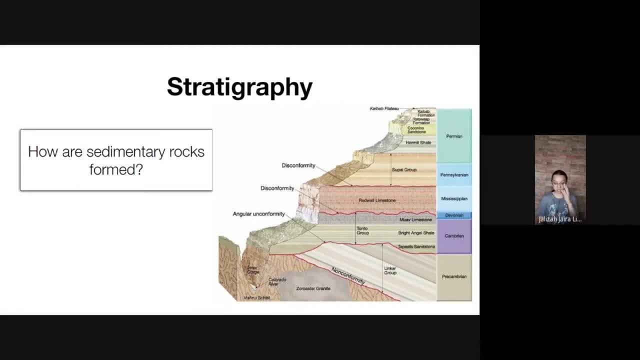 this particular, these different layers, were subjected to those processes and more. Because of that geochronology, which is the uh, the biological history of rock formations, and that the order, it's possible that the order can tell us about the age of the layers. 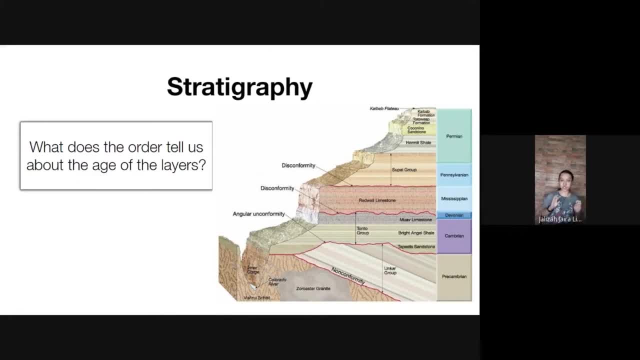 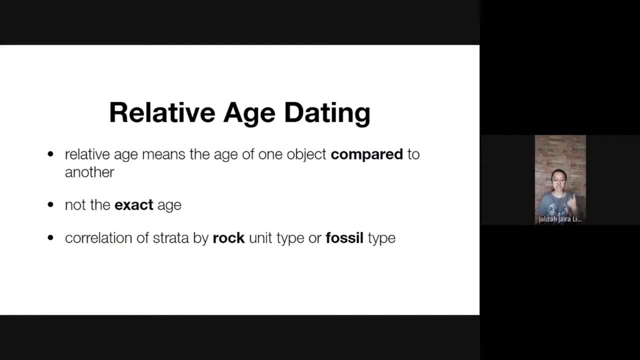 So there's a possibility that maybe the older ones are found at the bottom, the younger ones are found at the top. So with that we go into the prospect of relative age dating. So we try to understand here the age of objects when compared to another object. 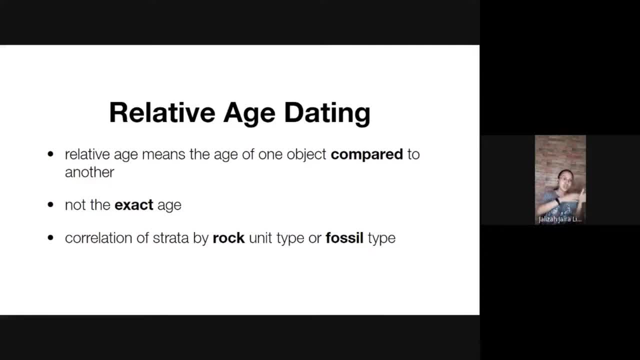 which is in this case. we're trying to compare the layers of rock with another layer of rock. It may not tell the exact age, though, but at the same time we can correlate the rock layer based on the rock type that is found there. 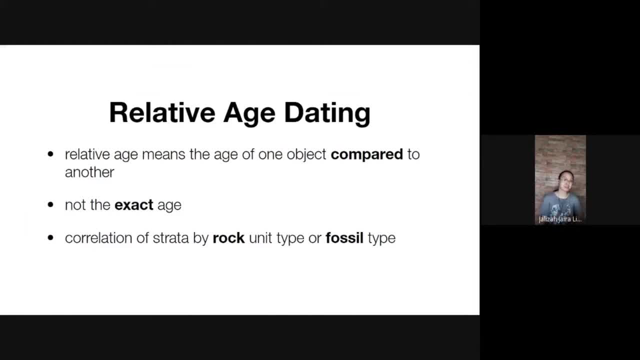 or in the fossils found in sedimentary layers. Now let me ask a question. first, Why is it so important to find out the actual age of objects? Why are we not satisfied with an estimate, or why are we not satisfied with relative age dating? 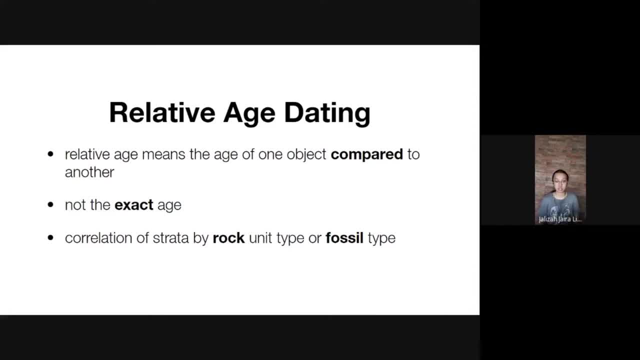 We actually have other methods of dating as well that are more accurate. I'm pausing so you can answer the question Right, because in science we try to pursue the truth, And so with that we want to have the most correct information that we have, such that we can. 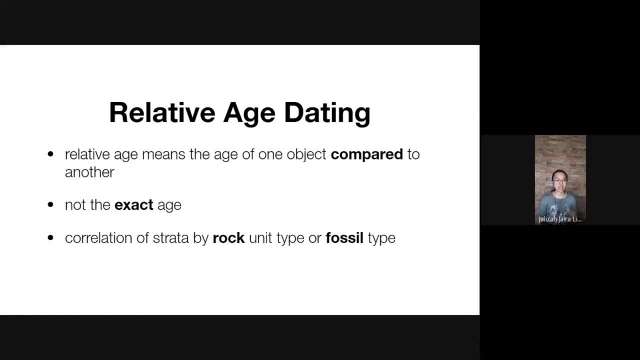 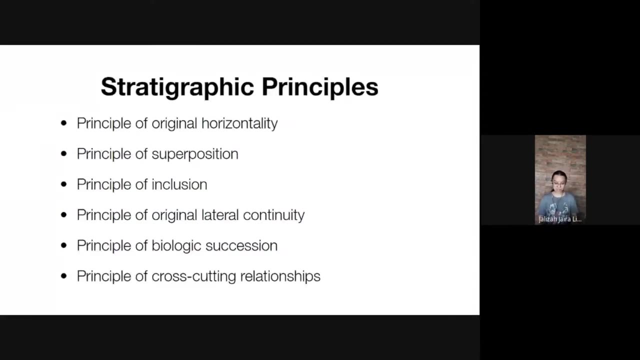 pass on this truth to the next generations. And what Miriam value is that You got it. It's the truth. So eventually, it's also important that you, as yourselves, live out your own truths, regardless of what anyone could say. So there are. these are the different stratigraphic principles that we will try to discuss for this video. 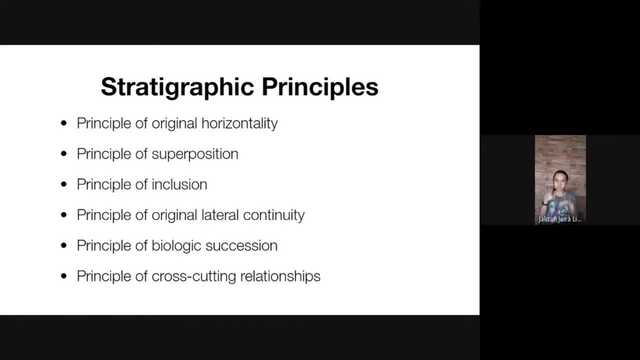 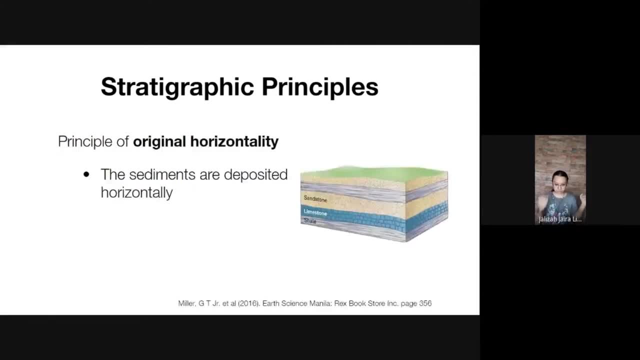 Don't worry, I know they look a lot, but we're going to try to slow down and try to discuss it as well as I could, So let's get on with it. First we have the principle of original horizontality. 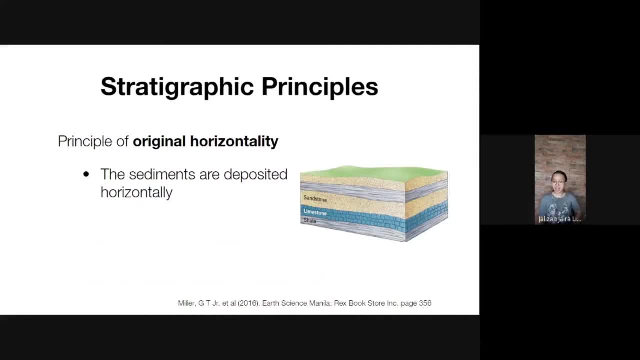 What the principle of horizontality will tell us is that sediments are deposited horizontally- And that's pretty much it- such that one layer will be found in a horizontal layer. So eventually, all the different sediments are found in one layer. So this is actually what it looks like. 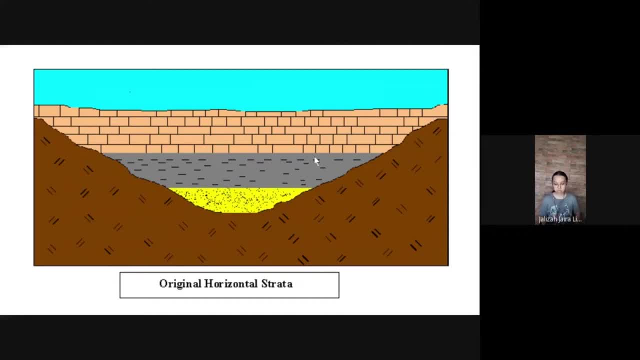 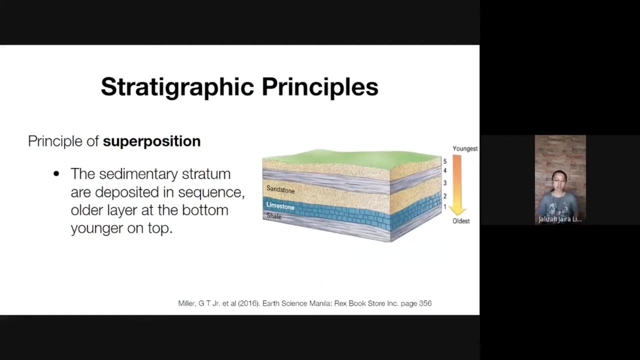 So that such that this layer is different from another, This layer is different from another, And then, finally, this layer is different from all the other two layers that were found Up. next, we have the principle of superposition. So the principle of superposition tells us that different layers are deposited in a sequence. 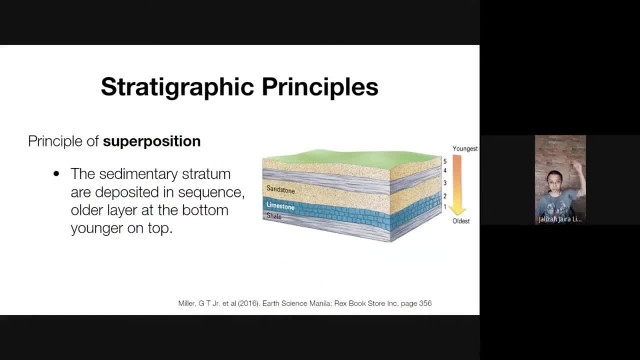 And that the older layers are found at the bottom, The younger ones are found at the top. So with that, let's look at our layer. here We have sandstone, limestone and shale. Based on the principle of superposition, shale would be the oldest. 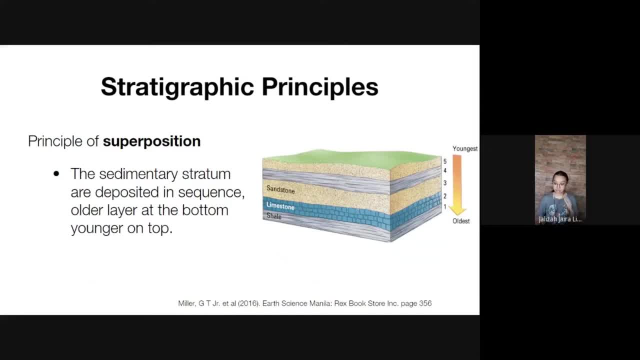 Afterwards limestone And finally, the youngest among these three layers is sandstone. Now, if ever we're going to go forward, the second layer is the second oldest And finally, the youngest layer would be the sandy structure right here. Easy enough, right? 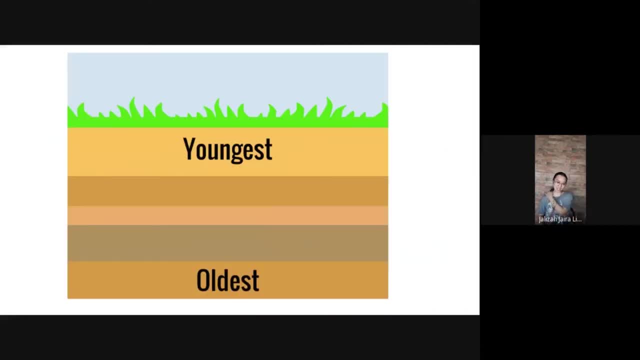 It's very good. Now again, just to emphasize, when it comes to the principle of superposition- oldest layer at the bottom, youngest layer at the top- Because this particular principle will oftentimes be used in experiments and scenarios that we will discuss all throughout this module. 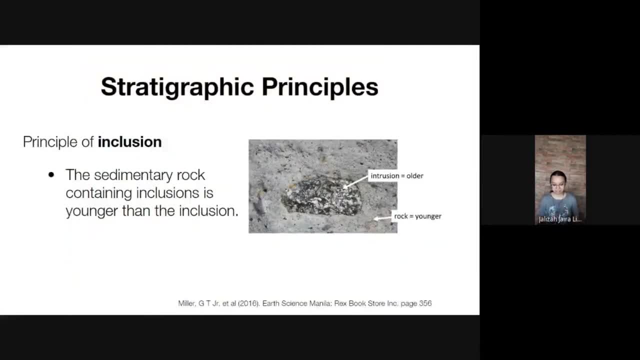 So it's best to understand this one. Up next we have the principle of inclusion. So the principle of inclusion, Inclusion will tell us that rock layers containing inclusions are much younger than the actual inclusion. So with that we have this rock example right here. 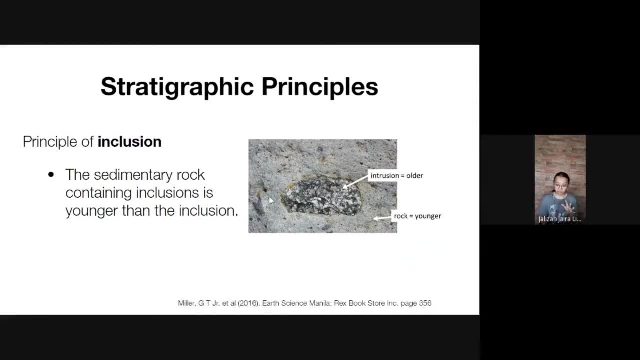 The rock in the middle is the intrusion, The rock on the outside of it is oftentimes a sedimentary rock, And that the inclusion layer is older than the rock that it is embedded onto. So, again, the intrusion is always older Then the rock surrounding it. 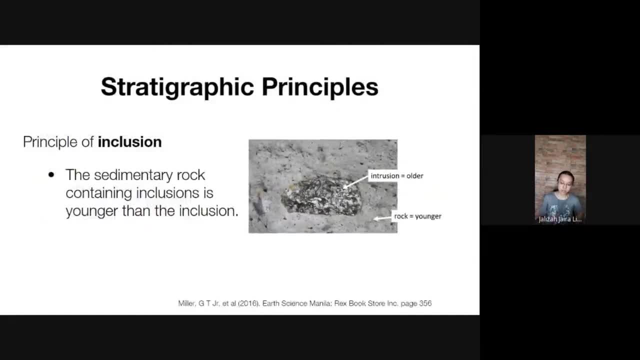 Now, these are some examples, But, Ms Lin, why did that happen? There is also a possibility that the intrusions have already existed and that rocks have gradually started to deposit around them and eventually surround them. So that's one hypothesis for that. 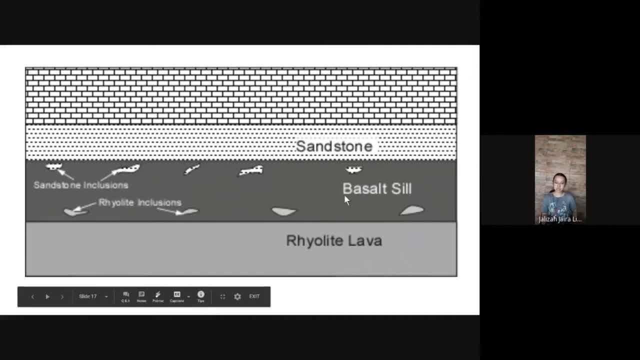 And this is a short example. Okay, let's look at the basalt silt and the rhyolite lava. Just this layer first. Ignore the sandstone, ignore the topmost layer Between the basalt silt. let's look at the basalt silt. 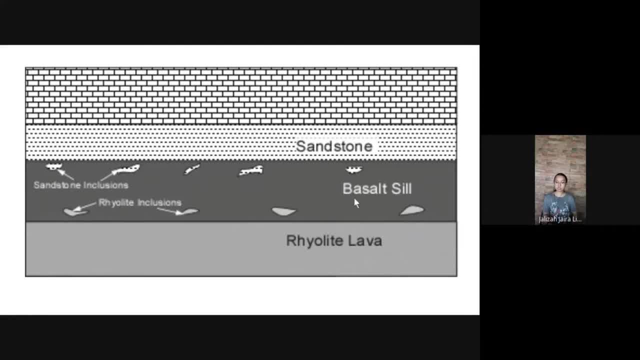 It includes inclusions. The basalt silt will have inclusions of rhyolite and sandstone. So with that which is older, the basalt silt or the rhyolite lava, So with that based on the principle of inclusion. 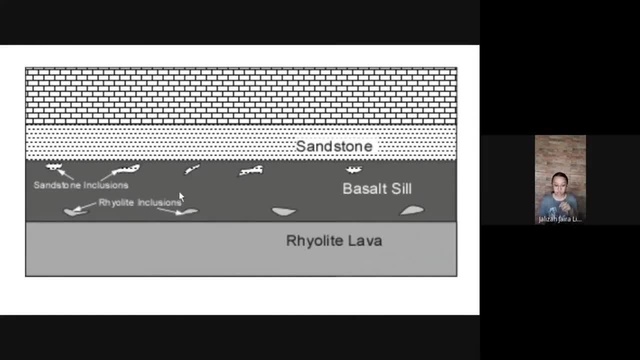 the rhyolite is older Then the basalt silt. What about this one? Let's look at the sandstone right here and the basalt silt, which is older. Based on the principle of inclusion, the sandstone inclusions are older than the basalt silt. 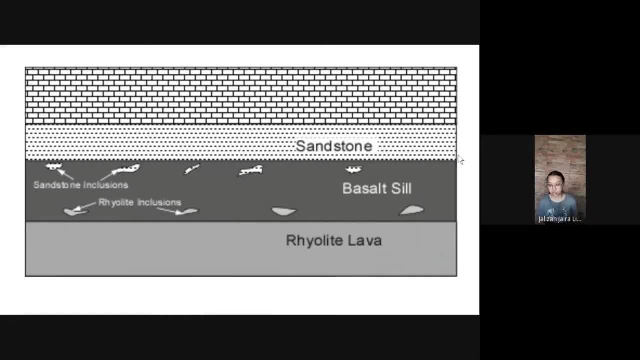 The story, possibly for this one, is that basalt is actually made as an example of igneous rock, So chances are these are at the. these two layers were actually together, But eventually magma may have intruded and eventually enabled these inclusions to happen be made. 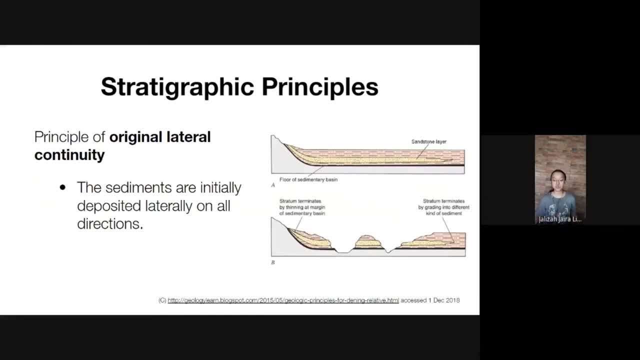 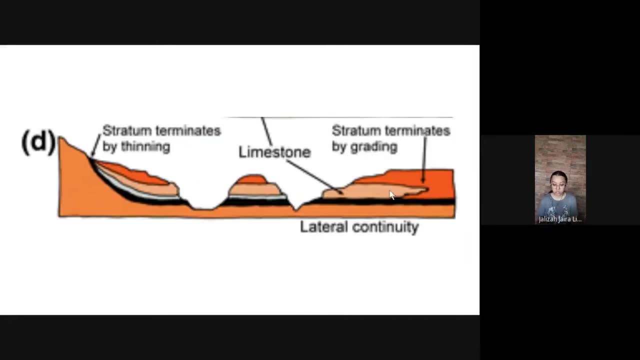 You also have the principle of original lateral continuity. What this principle will tell you is that sediments are initially deposited laterally on all directions. So with that, regardless kung magkaroon ng erosyon, regardless kung magkaroon ng erosyon. 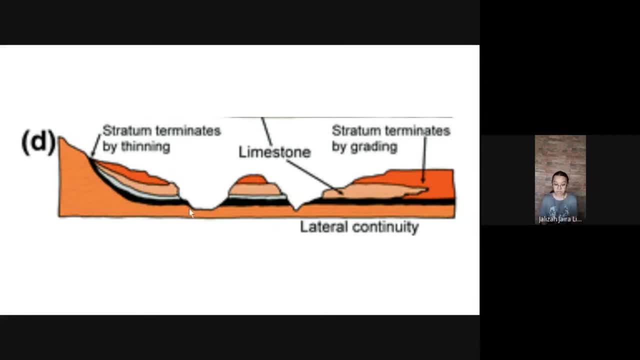 these two layers are still of the same age. So this orange is the same age as this orange, This peach is the same age as this peach, This white is the same age as this white, and so on and so forth, Because originally they have. they were deposited in one horizontal layer. 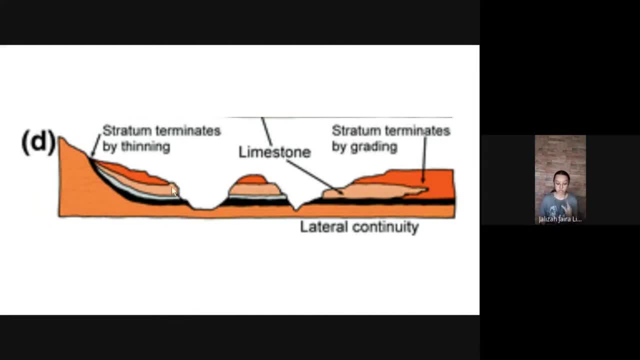 but because of different events surrounding the earth, chances are nagkaroon ng ganyan. So we have to follow the principle of lateral continuity to determine the relative age of these rocks based on kung saang layer sila naghagita. 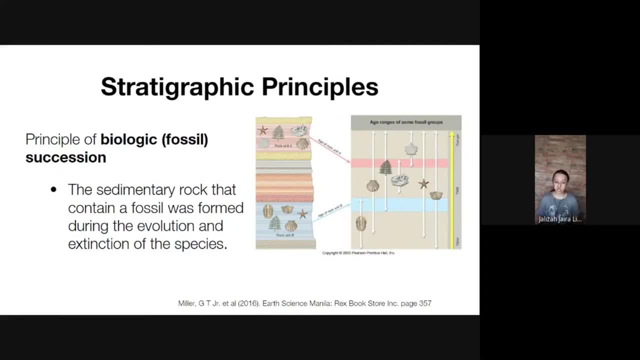 So we also have the principle of biologic succession. So what the principle of biologic succession will tell us is that sedimentary rocks that contain a fossil were actually formed during the evolution and extinction of these different species. What does that mean? It means that if you see a sedimentary rock and you can't determine its age, 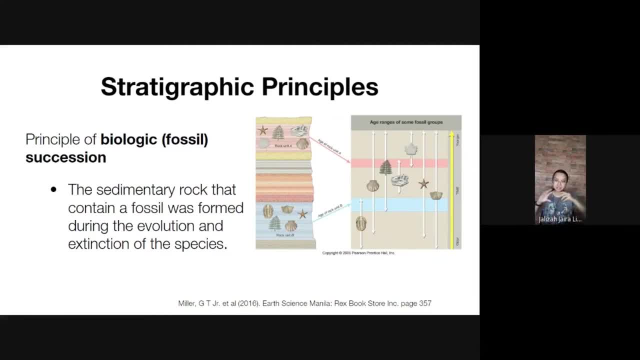 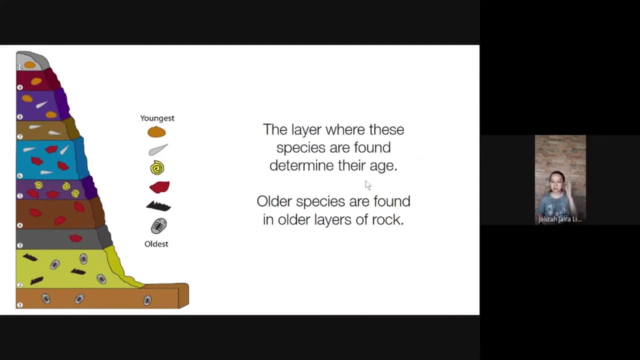 but you find the fossil in it. chances are the age of the fossil will actually give you a clue as to how old the sedimentary rock is. That's because we have these index fossils Now at the same time. again, the layer where these species are found will oftentimes determine their age. 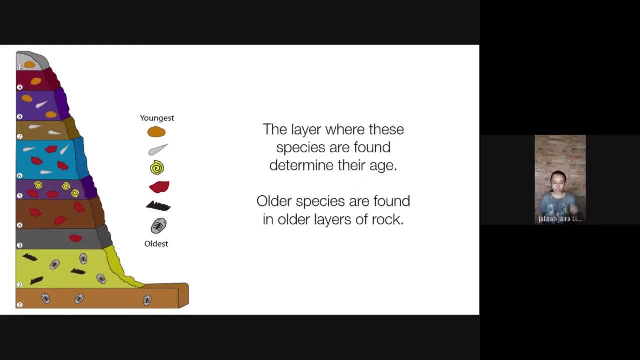 In the same way, older species are found in older layers of rock, just like what you would see in this example right here. Let's look at the clams. Where do you find the clams? Which layer? There are 10 layers all in all. 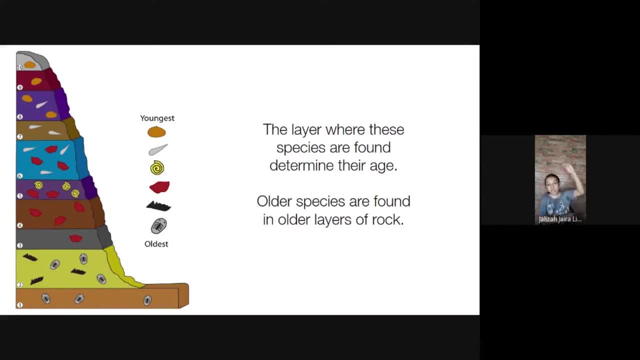 So you find it in 8,, 9, and 10, which is on the topmost, And usually the topmost layers are usually the younger ones. What about the trilobite right here? This trilobite, where can you find it? 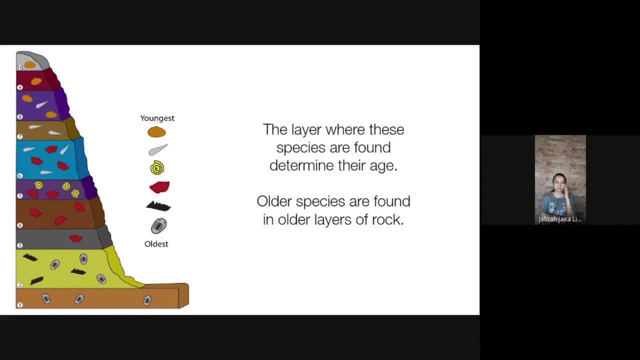 It's found in the bottom most layers, primarily 1 and 2. So in a way we can actually utilize fossils to tell us the age of rocks, or rather the relative age of rocks. We also have the principle of the age of rocks. 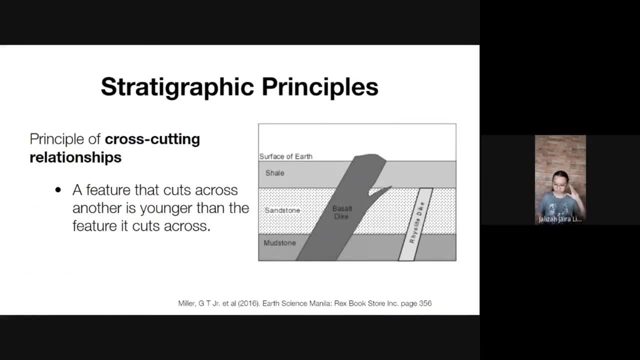 Cross-cutting relationships. So the principle of cross-cutting relationships is a little bit more tricky, Because what we have here is that these are usually features that cut across another rock And that these features- this cross-cutting feature- is usually younger than the features that it cuts across. 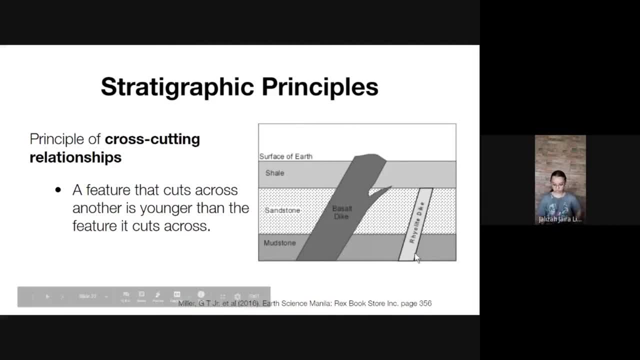 What does this mean? Let's look at this one. We have mudstone, sandstone and shale, And then we have cut-ups of basalt and rhyolite. Now let's look at this one. Let's focus first on the rhyolite dike. 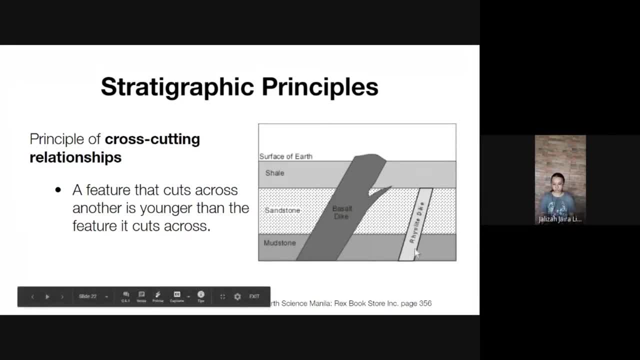 This feature right here that cuts across the mudstone and the sandstone According to the principle of cross-cutting relationships. the rhyolite is younger than the sandstone and the mudstone Because that's what it cuts across Again, while we focus on this one. 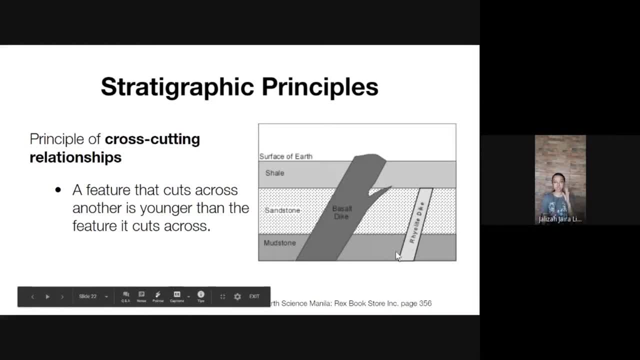 rhyolite is younger than sandstone and mudstone because it cuts across it. Chances are, rhyolite is also an igneous rock, So because it was formed from magma, it's possible that there was a vent here and eventually it got in there. 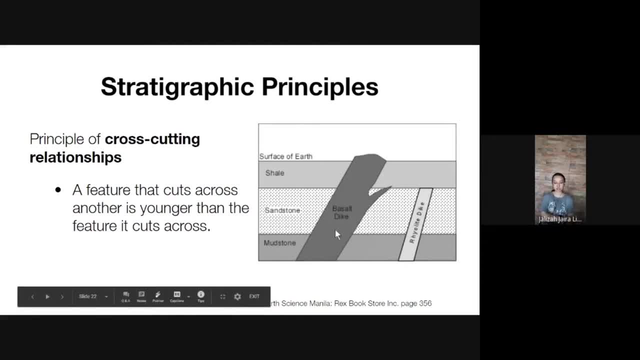 That's why it formed here. What about basalt? Let me ask you the question: Is basalt younger than shale? Is basalt younger than sandstone? Is basalt younger than mudstone? The answer to all those questions is yes. 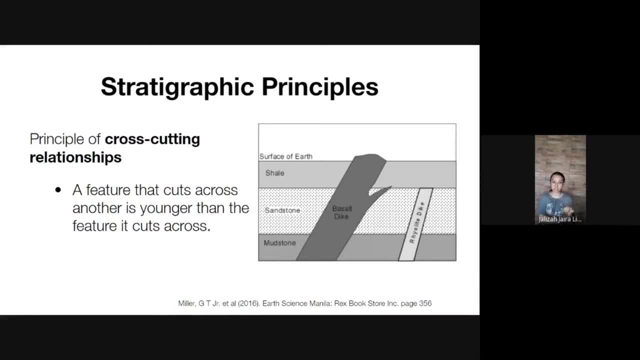 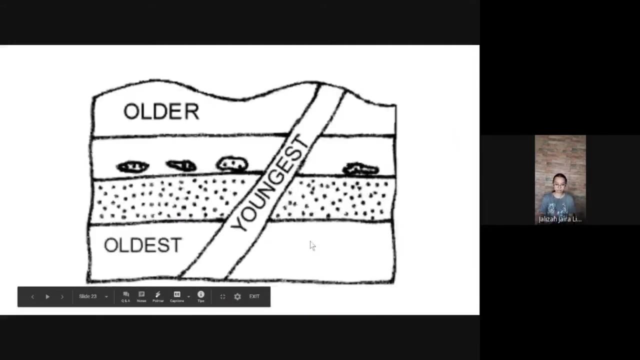 Because of the fact that, according to the principle of cutting relationships, the feature that cuts across is always younger than the layers that it cuts to. So, in this case, basalt is younger than shale, sandstone and mudstone. Remember, the one that cuts across is always the youngest. 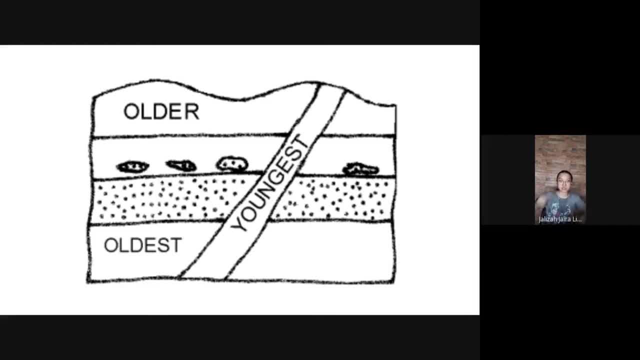 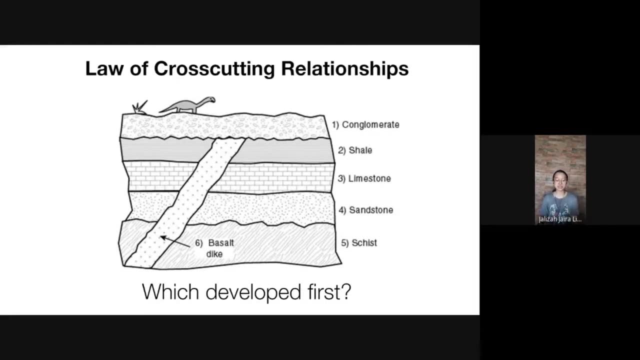 Just like how we have younger kids. Have you ever had younger siblings And that? oftentimes they cut into the conversations because I'm just kidding. Love your younger siblings, I definitely love mine. So this is just a short exercise for the law of cross-cutting relationships. 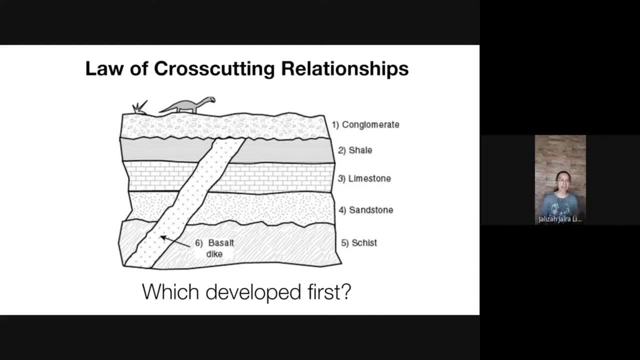 Which developed first. I will let you have this for a few seconds, So while you solve this, me and my puppet will dance. I'm getting hot here. Okay, Now going back. So which developed first Among all the structures which developed first? 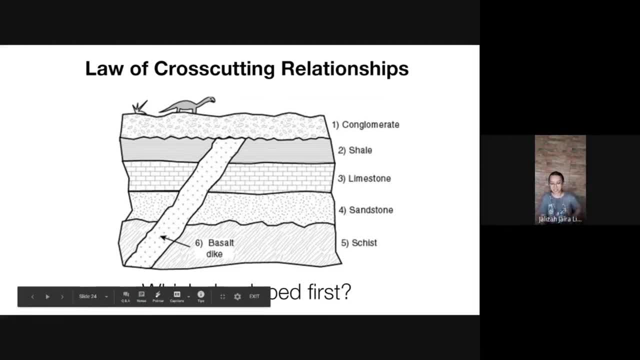 If you answered schist, you are correct. It's actually schist. So here we also have to follow the principle of superposition. You always have to apply all the other principles that you have learned, So the oldest one here is schist. 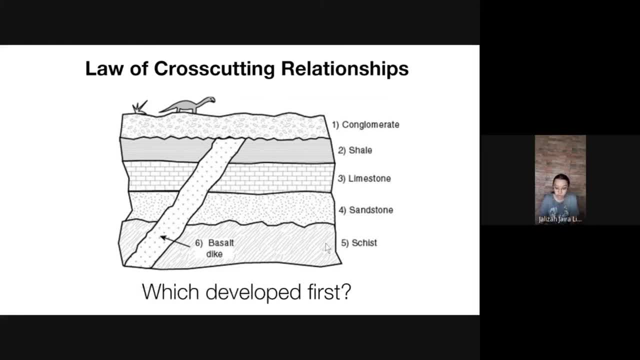 Up next is the one that formed. next is your sandstone, After sandstone, limestone, After limestone, shale, Now after shale, which is the next formation. The next formation is your basalt dike And then, after the basalt dike, 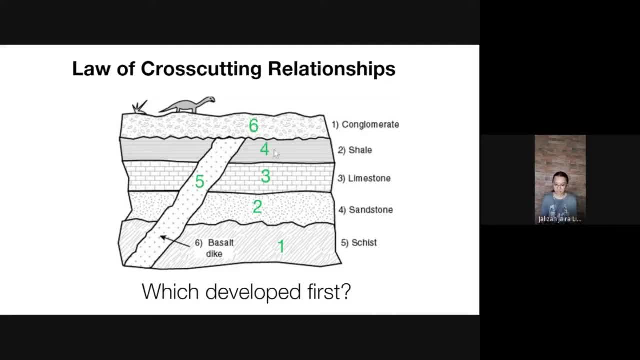 it's actually your conglomerate. So these are the actual progression of things. Okay, So remember dahil nag-cut siya dito at hindi siya umabot sa conglomerate basalt is only younger than these four layers, but not the conglomerate layer. 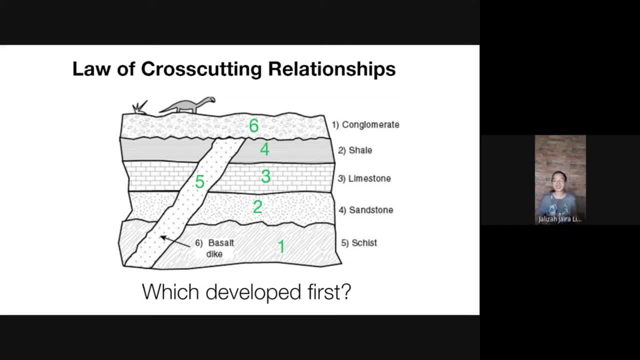 Kasi hindi naman niya naepalan, hindi naman niya na-cut across yun. So there are two, there are many principles that you have actually observed here. First is the principle of superposition, principle of horizontality, principle of lateral continuity. 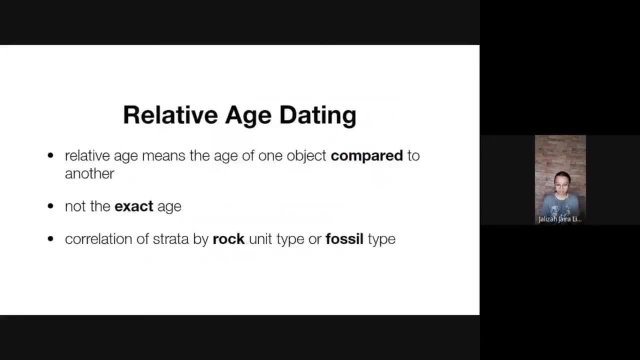 and then principle of cross-cutting relationships, So relative age dating. again, they just try to tell us about the age of one object to another. So relative, there's always comparison. Now, again, it does not tell us the exact age and that we usually correlate the strata. 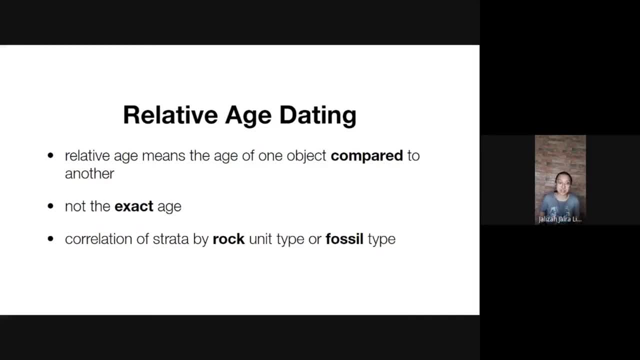 the age of the strata, based on the rock type and the fossil type. So again, you don't really have an exact age for relative age dating. So just another fact is that it's usually dominated by your principle of original horizontality and superposition. 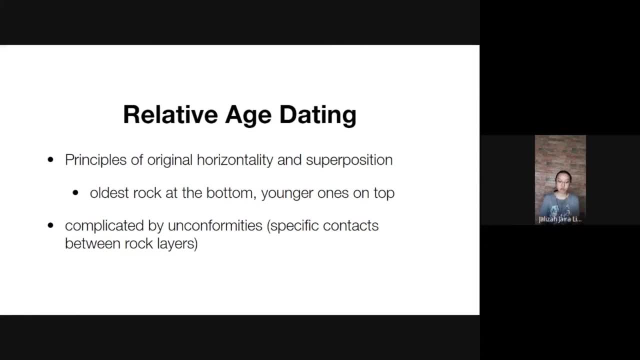 So ito yung pinaka-importante that you should know: Older rocks at the bottom, younger rocks at the top. However, these are oftentimes complicated by unconformities. When we say unconformities, these are actually erosion events that can actually compromise yung pagkakapatong-patong ng mga bato. 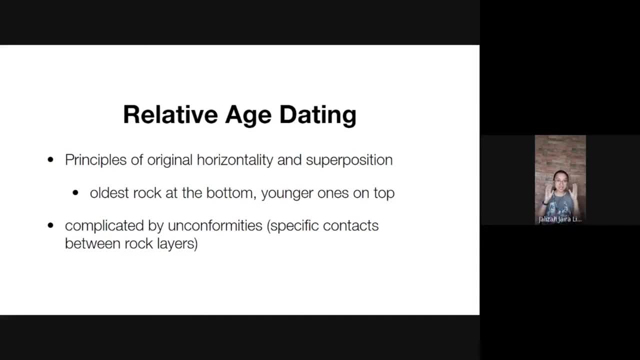 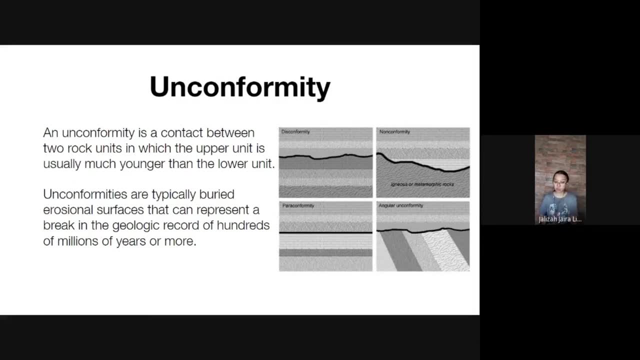 Pag na-compromise, yung pagkakapatong-patong ng mga bato. hindi natin alam kung sila nauna. So an unconformity is a contact between two rock units, like here. The unconformity is the deep black lines and that they usually tell us that the upper unit is much younger than the lower unit. 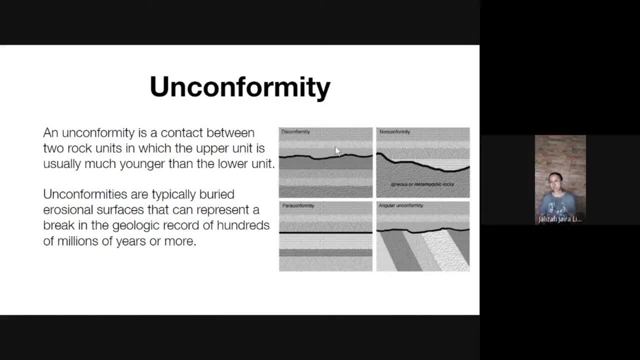 Ang problema dito is that it's much younger, So chances are may layer of rocks Na nawala Nagkaroon ng erosion event between these two. So a lot of history has already been lost. A lot of the story has actually not been told yet. in that sense, 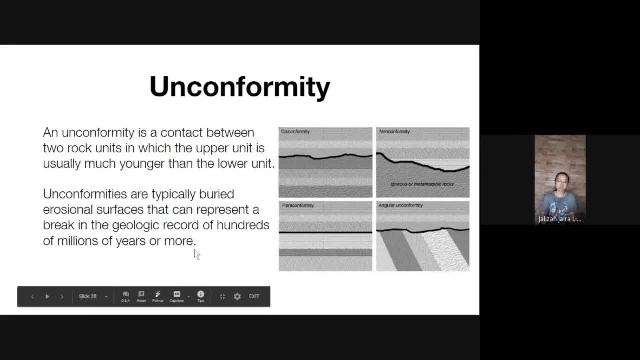 And unconformities are usually buried on erosional surfaces And that the problem with unconformities is that it means that there's a break in the geologic record. It means that may rock layer na naeroad and it has been gone. 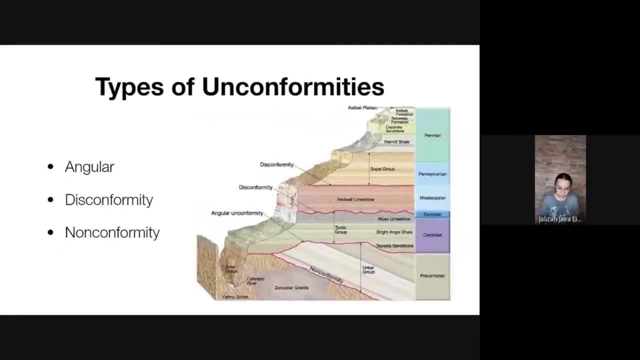 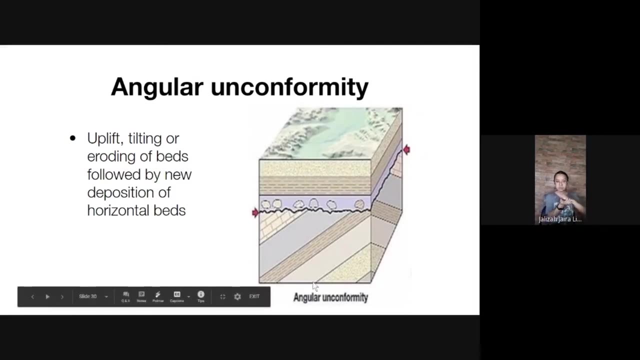 It has been well eroded. There are three types of unconformities. We will talk about angular, disconformity and nonconformity. When it comes to angular conformity, ang nangyayari dito is that there's an uplift of the rock beds, eventually followed by a deposition of horizontal beds. 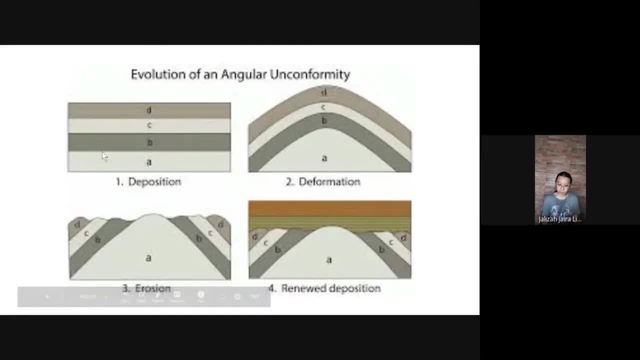 So ano yung story niyan? First is deposition And eventually nagkaroon ng deformation or tilting, Nagstart siyang mag-tilt. Bakit siya nag-tilt? Either nagkaroon ng fault sa rock layers below it pa, or there's some sort of event that made it happen that way. 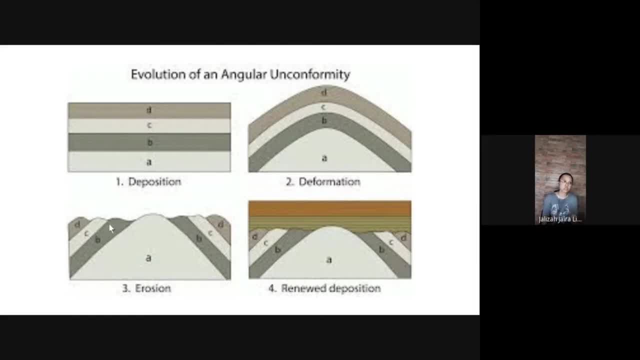 Afterwards nagkaroon ng erosion. Now, erosion, of course, can be subjected or there can be caused by different factors. However, ang problem dito is that nagkaroon ng bagong deposition on top of the original rock layers, resulting to angular unconformity. 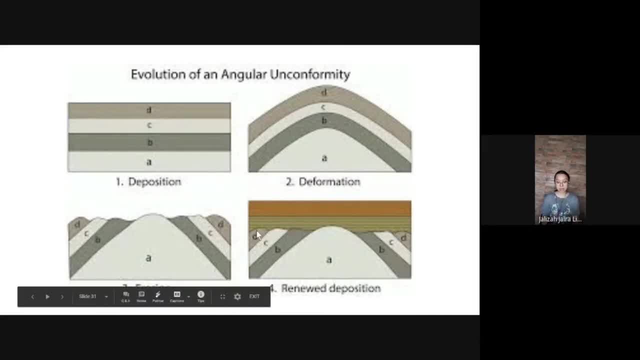 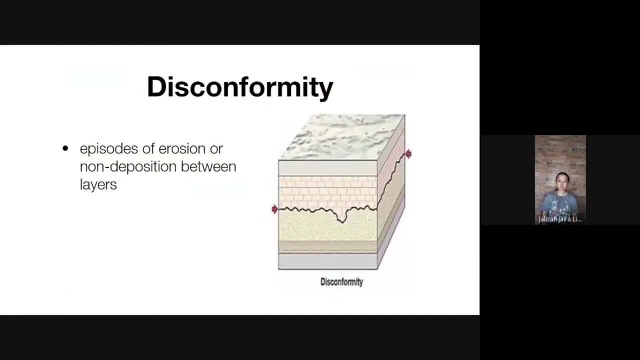 We say angular unconformity because hindi sila paralel sa isa't-isa, More or less there's a tilt to it. So we also have your disconformity, which is episodes of erosion or non-deposition between layers. 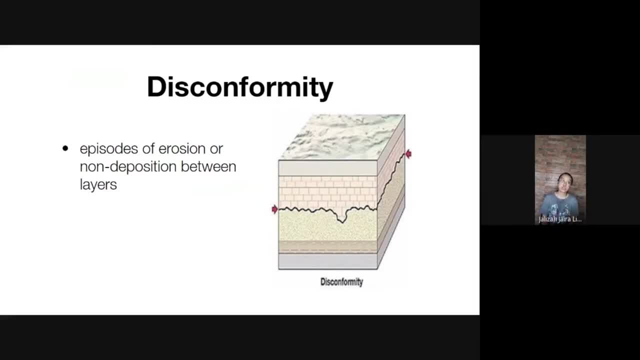 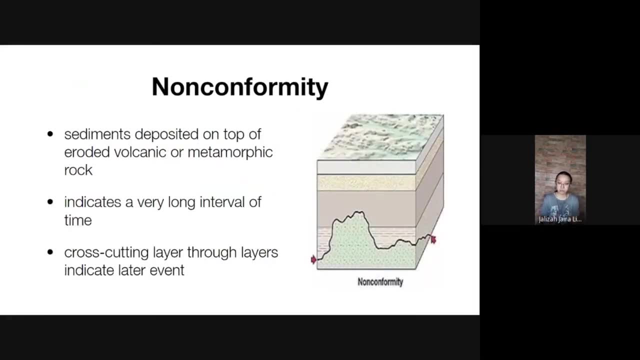 This actually usually occurs between two sedimentary rock layers, wherein magkaiba sila, We also have nonconformity, which actually is oftentimes between sedimentary rock layers. So we have sedimentary layers and volcanic rock layers, be it igneous or metamorphic rock. 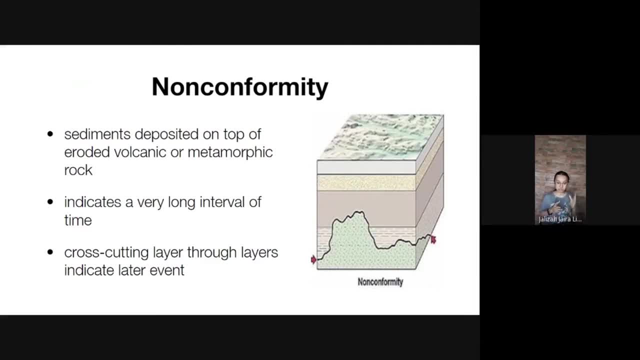 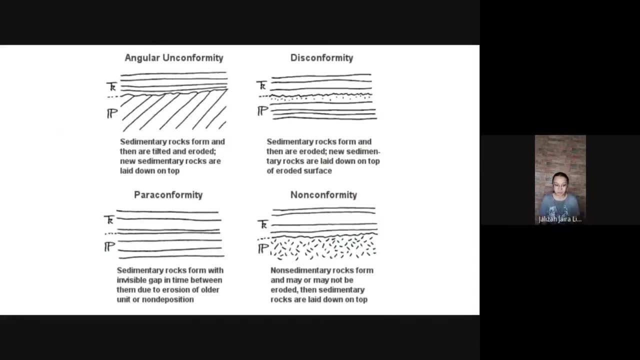 And that nagkaroon ng cross-cutting by the metamorphic or the volcanic rock into the sediments. So to further simplify those explanations again, disconformity is when sedimentary rock layers form, then are eroded and eventually new sedimentary rock layers form on top of them. 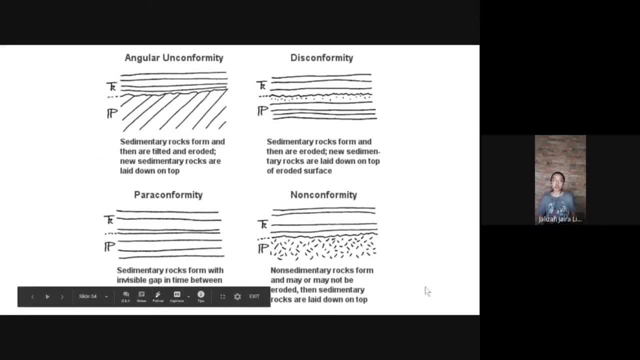 Nonconformity is when non-sedimentary rocks or igneous or metamorphic rocks may form and they also get eroded and then eventually sedimentary rocks start to form on them. So again, these are usually categorized by erosion episodes in between rock layers. 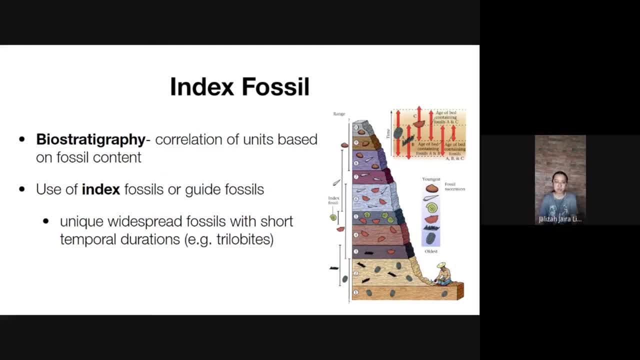 So this is the last part of the video. If you want to take a break, don't forget to pause, get some water. I know it's a very long video, but remember you are in control of your pace. You don't need to finish your video in one go. 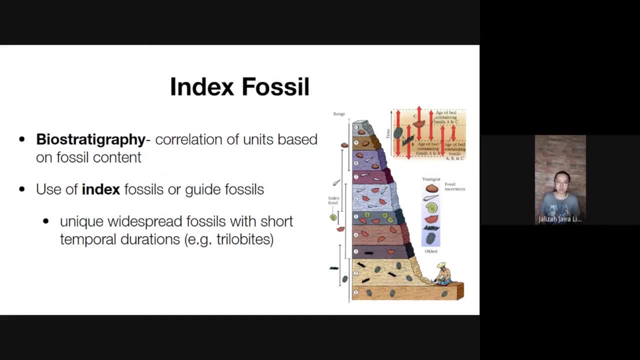 You can always just take pauses. I'll be adding timestamps as well, don't worry. So we go back to your index fossils. They are actually very useful in a field called biostratigraphy, which actually tries to correlate the units based on fossil content. 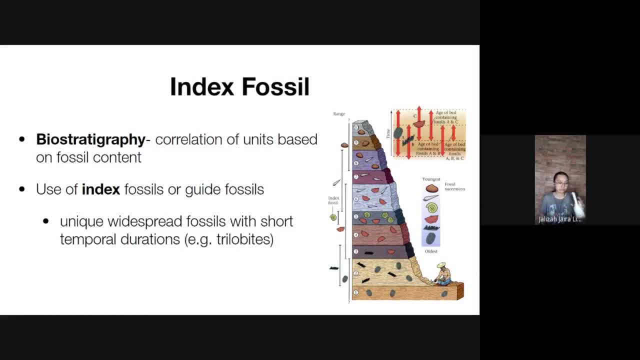 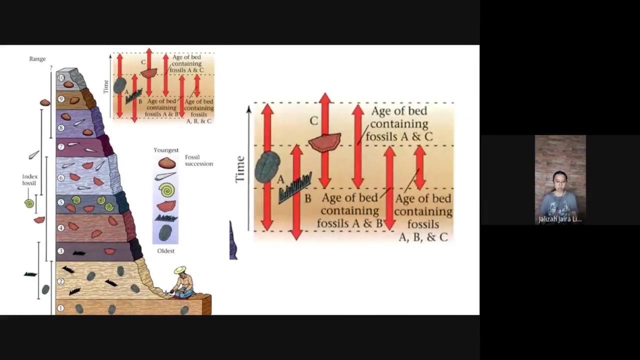 So different rock units according to fossil content: Index fossils actually tell us about the time or the age of the rocks that are actually present, Or rather, index fossils tell us a lot about the rocks that they are embedded in. So actually just this particular picture right here can actually show you basically. 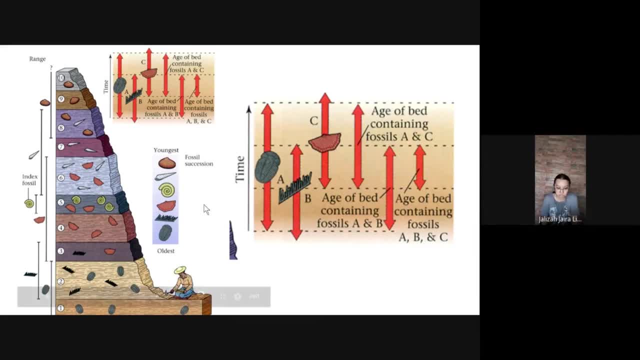 this basically follows the principle of biologic succession. But what index fossils do is that they can actually tell you when certain events have happened, such that as to why species went extinct, based on the rock layers as well. So we usually utilize the index fossils to actually tell the age of your rock layers. 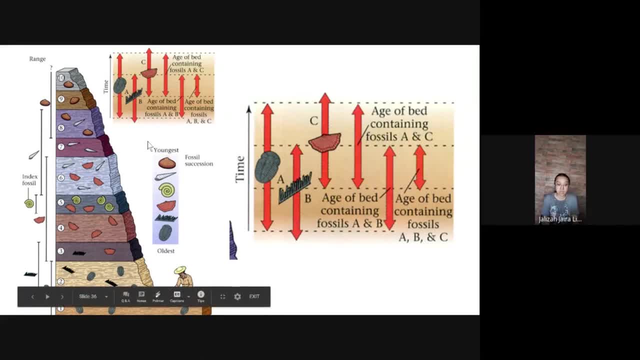 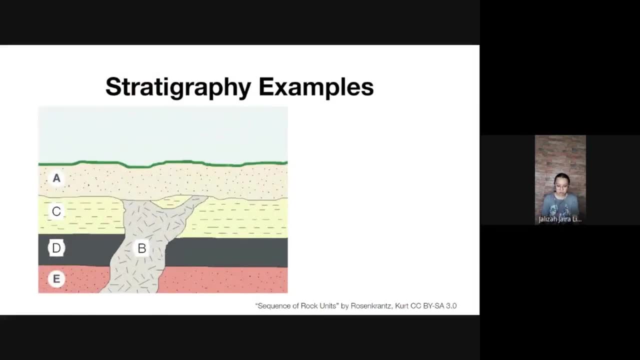 based on kung gaano katanda yung index fossils, As index fossils can actually be subjected to radiometric dating. So here are more stratigraphy examples for you to work on. So we're going to try to understand the formation sequence. So ano ang nauna. 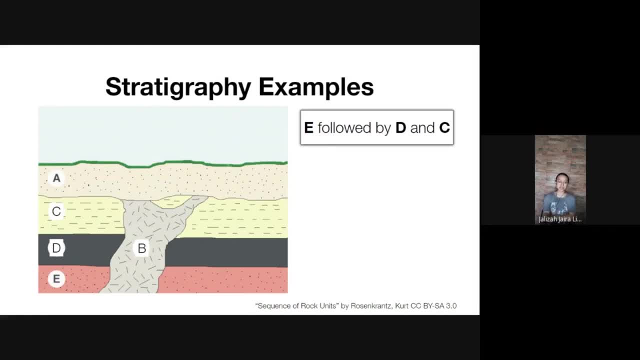 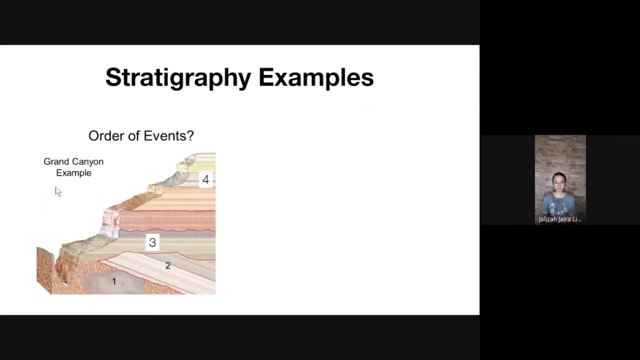 Letter E and then followed by D and then C. Then what comes next? Letter B, karoon ng crosscutting episode by B. Then there is also some erosion, because hindi siya single layer lang. And then up next there is deposition by rock layer A. 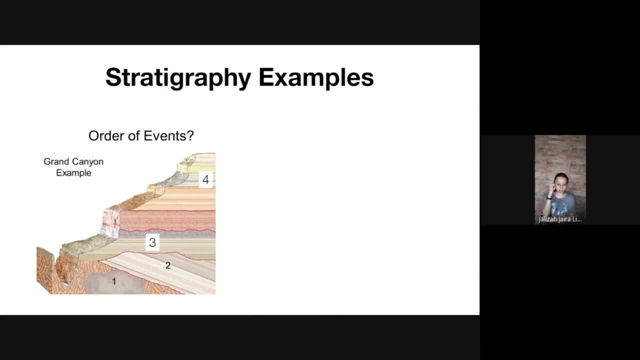 So how about this one Between 1,, 2,, 3, and 4,? what are the order of the events? Formation first of 1, after certain geologic events, Deposition by 2,. but here nagkaroon siya ng angular unconformity. 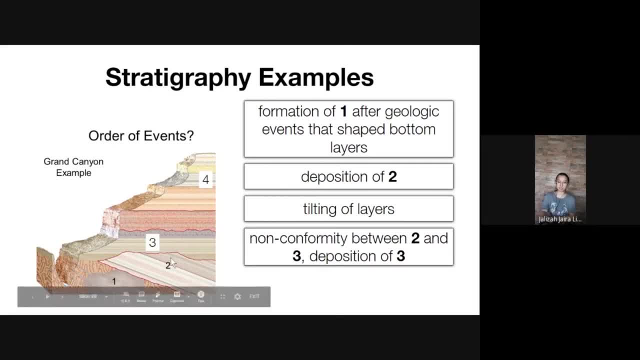 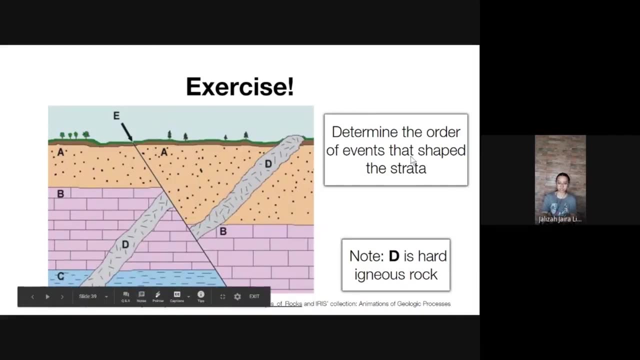 Eventually the layer started to tilt And then nonconformity between 2, 3.. So there starts the deposition of 3.. And eventually the deposition of layer 4.. So here's another exercise for you: Still determine the order of the events that shape the strata. 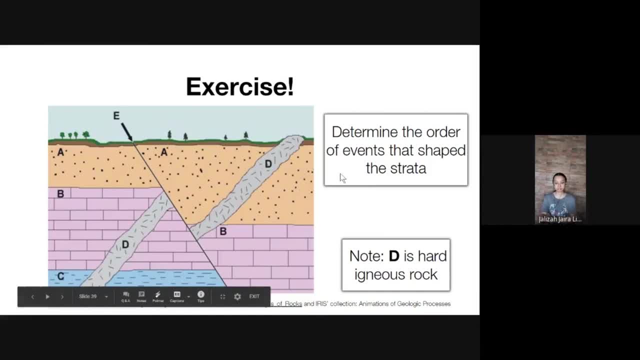 Take note that D is a hard, igneous rock. Ah, in-flash ko agad yung answer, Sorry, So take the time first to try to solve it on your own, And then the answers are actually found in the next slide. So first muna is letter E. 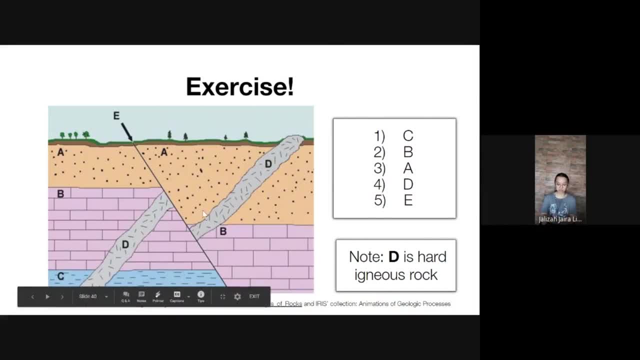 So nagkaroon muna ng earthquake. By the way, sorry, The first event is actually C. The first event is C, Followed by the cross-cutting of D. At this point, medyo sabaw na ako. The first event is C. 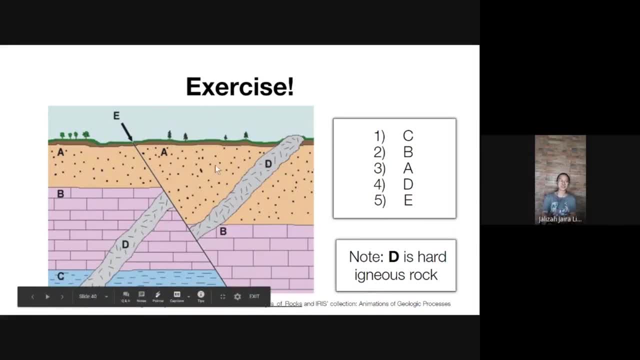 Followed by the formation of B, Followed by the deposition of A, And then the cross-cutting of D And then, finally, the faulting done by E, As E actually cuts across all the 4 other layers. I am so sorry, It's been a long day.